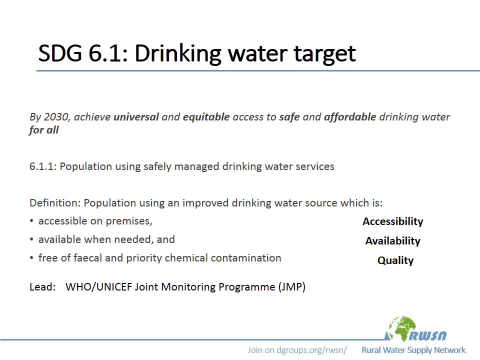 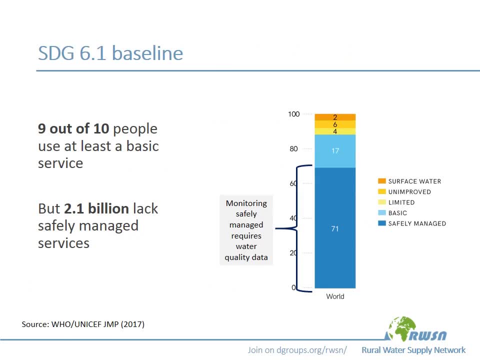 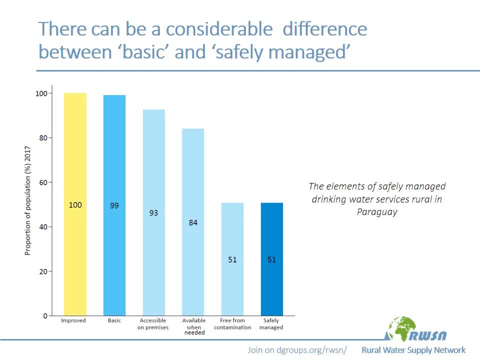 universal and basic 99% so only 1% of the population lack basic services in rural Paraguay and whereas if we look at the elements of safely managed so 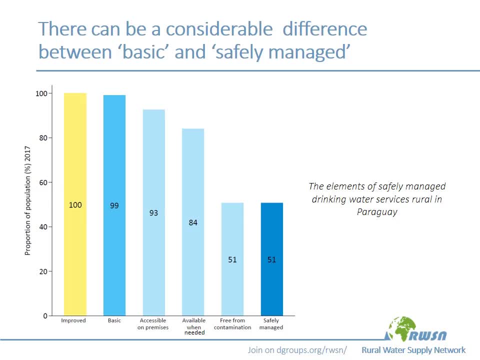 accessible on-premises available when needed and free from contamination you can see that there are big drops but the most pronounced drop of all of those is some is the freedom from contamination which is based on data from one of these household surveys 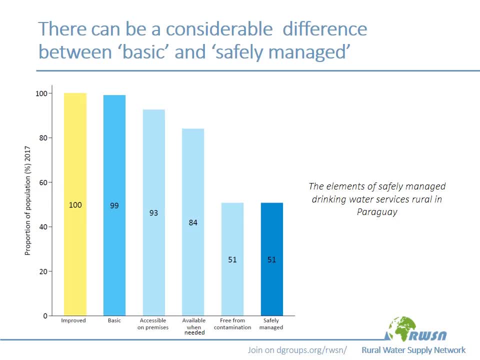 and we take the minimum of those three elements and to get safely managed which is this 51% there so half of the population of rural Paraguay use safely 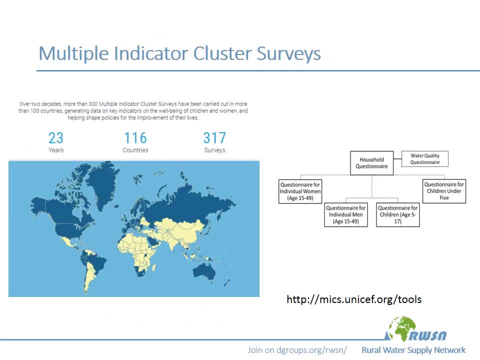 managed drinking water services so what our mix surveys mix is a multi-topic survey covering a wide range of issues about children and and the well-being of 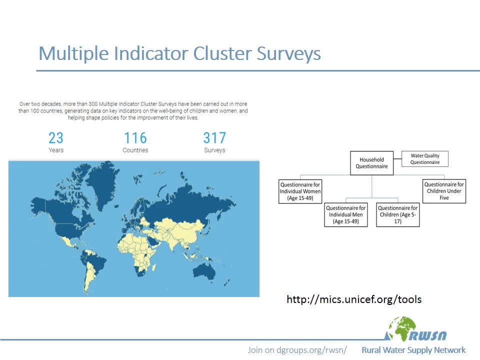 children and their families one of the really exciting new additions to mix has been the the new water quality module which is a very important part of the mix and as you can see here on the right hand side it's linked to the 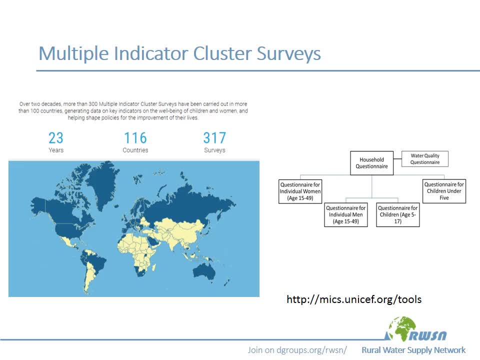 household questionnaire so we can find out information about households and then link the water quality directly to that mix have been conducted in a large 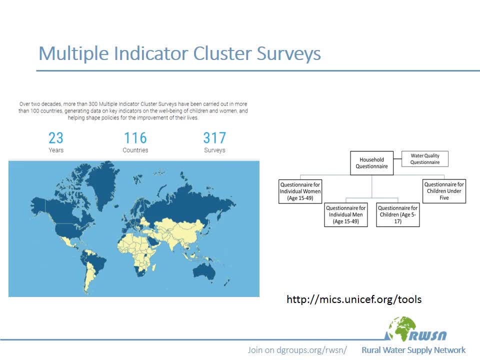 number of countries for over 20 years so what's the priority what should we measure the top priority at the global 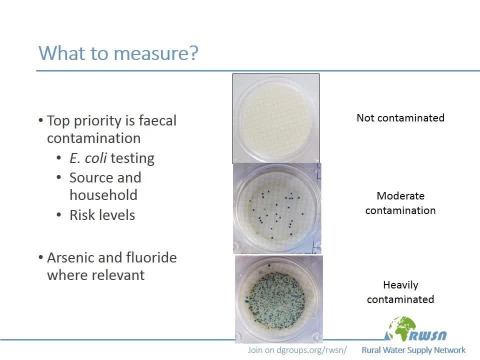 level is fecal contamination and the testing of e.coli or alternative flea thermotolerant coliform and in this module we focused on both the 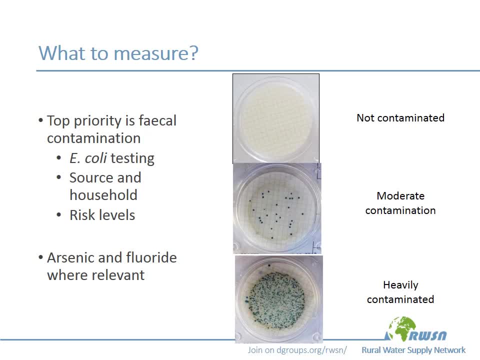 source of drinking water and a sample from within the household to try and understand any deterioration in water quality we're also looking at risk 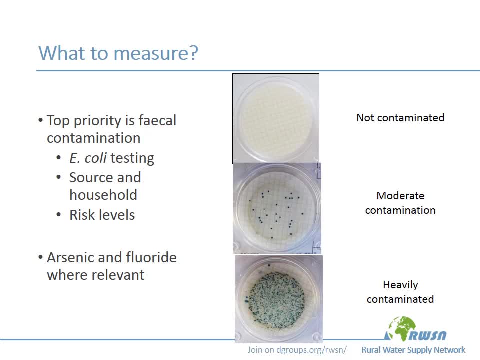 levels so trying to quantify e.coli and put it into risk categories so one to ten ten to a hundred over a hundred e.coli per hundred millilitres and then 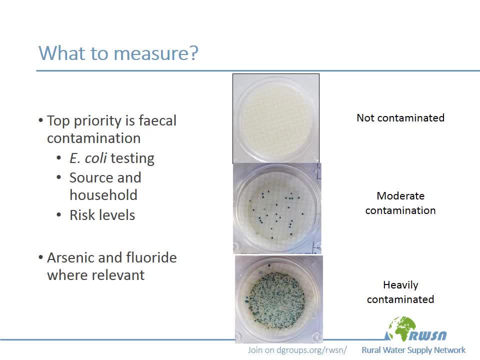 depending on on the country and arsenic and fluoride can be top priorities so for example in Bangladesh and Nepal 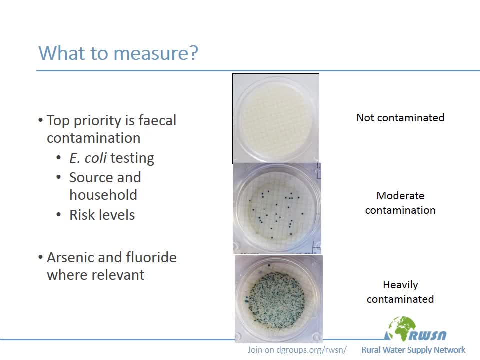 arsenic has been measured on the right hand side you can see some of the test results so this is using a compact dry plate where you can differentiate 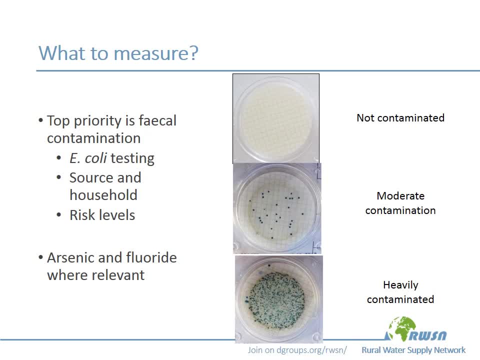 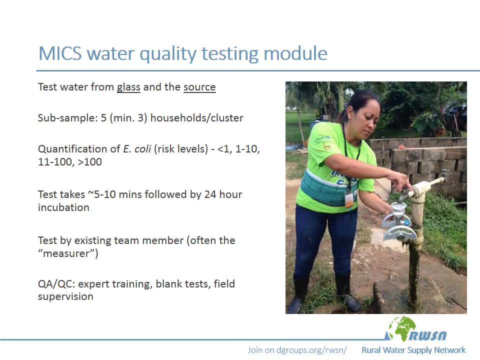 between not contaminated moderate and heavily contaminated samples the mixed water quality testing module as I said it tests water from a glass within the home so we start with that and then we 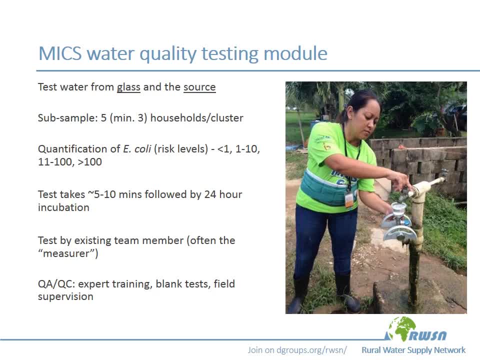 ask households to take us to the source of drinking water where they got that glass from so that's trying to understand the differences in water 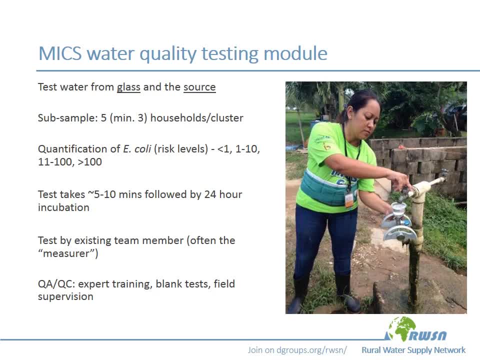 quality between those and a survey normally has somewhere between twenty and twenty-five households in a cluster and a cluster you can think of as sort of 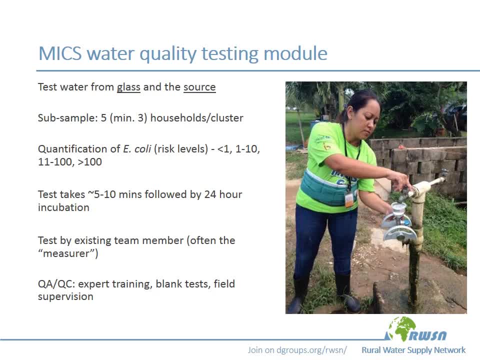 a hundred to hundred and fifty households and the reason for in the water quality module we reduce the number of households because it's a lot 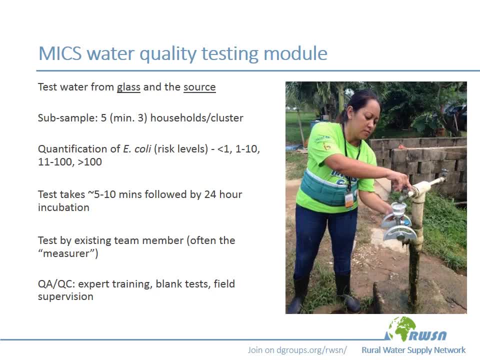 of additional work for somebody who has other during the survey. I mentioned the E. coli risk levels. The test that we're using is a modified 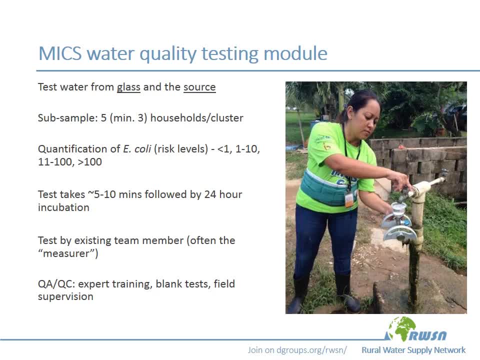 member infiltration method. It takes about five to ten minutes, followed by 24-hour incubation. 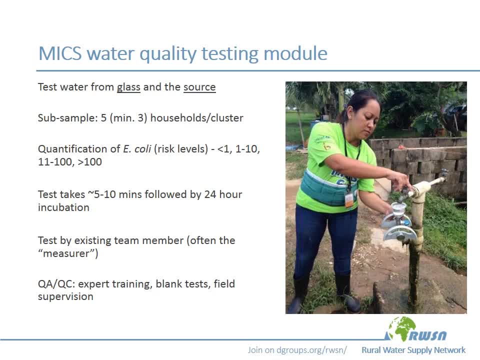 Importantly, the test is done by somebody who's already a member of the existing team, so it's not recruiting an additional person, which has obviously important implications for the cost. 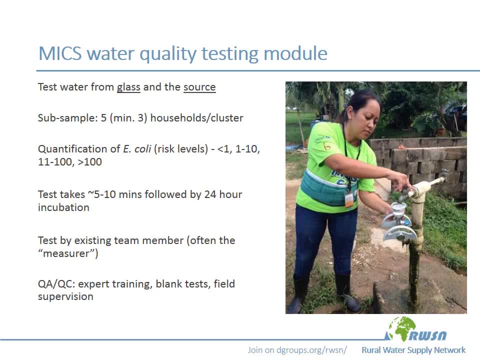 Usually, this is somebody who's responsible for anthropometry, so measuring children's heights, weights, etc. Another really critical element in this module is the quality assurance and quality control, where we work with national laboratories or line ministries to support the training of field teams, and the JMP maintains a pool of consultants who support that. We also focus very 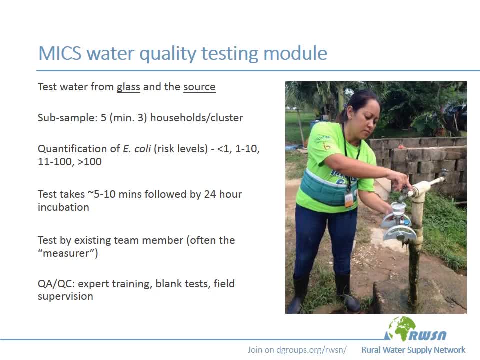 strongly on blank tests, so there's a blank test that we do. We do a lot of test in every cluster, and there's obviously field supervision, which is part of the survey. 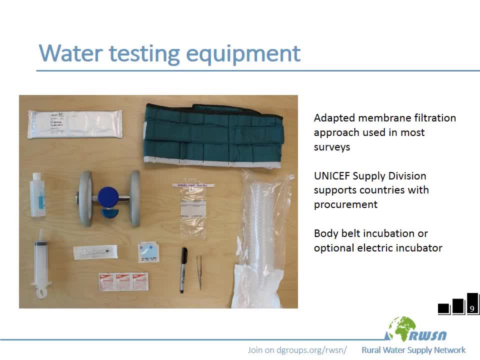 A little bit more about the kit itself. As I said, it's an adapted membrane filtration approach that has been used in most of the surveys, and you can see the manifold there in aluminium in the centre. 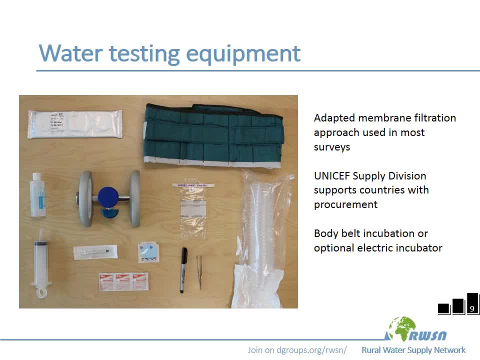 UNICEF's supply division has been supporting countries in procuring these. I think the other interesting 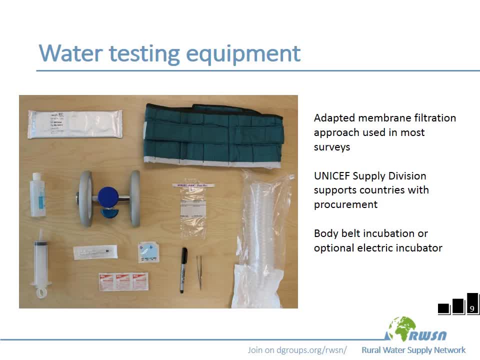 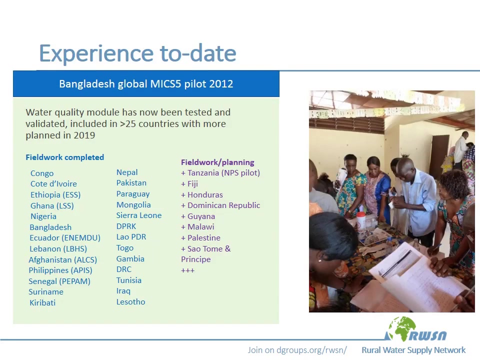 side of this... This is a millipore manifold and kit with sterile funnels, for example, is we're trying to find a way to allow people who don't have experience with water quality testing to do it reliably in the field. We've also used, as you can see in the top right, an incubation belt. This is to allow body temperature to incubate those compact dry plates, which is the E. coli testing plates, for 24 hours. There is an option of using an electric incubator, but in many contexts, that's more complicated than using an incubation belt. As you can see, we've had quite a number of countries using this module to date, over 25 now, with quite a few more planned in 2019. The other thing I'd like to point out is that quite a few of these surveys, the ones with acronyms in brackets, are countries that weren't supported directly by MIX, but are countries that have adopted the module and adapted it for their surveys. 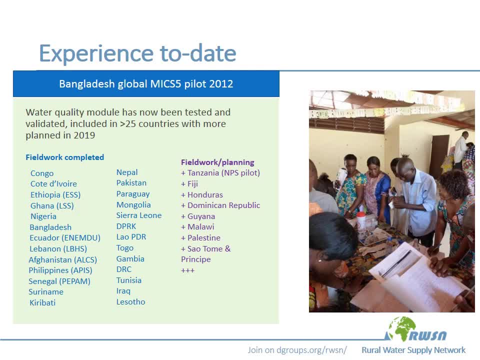 So, for example, in Ethiopia, Ghana and Ecuador, those were in collaboration with national statistical offices and with the World Bank. And there's a large number of surveys planned for 2019 and also for 2020. 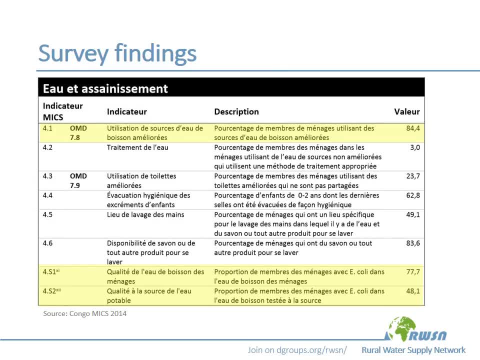 So what do we find in these surveys? Here's an example from Congo, where we can see in the top row, the proportion of the population using improved sources is around 84%. But if we look at the quality of water at the source, this indicator right at the bottom, almost half of the population use drinking water that is contaminated with E. coli. And by the time you get to the household and take a sample from the household, you can see that it's a glass of drinking water used by household members. It's three quarters of those samples had E. coli in them. So huge, huge differences between the source and the household. 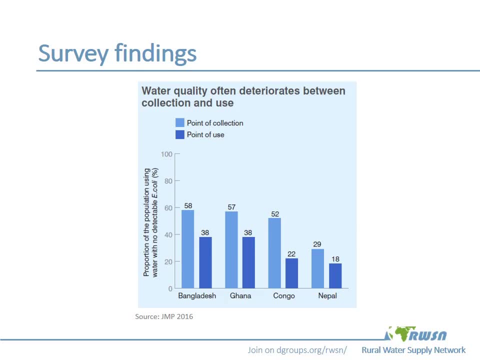 And we can see that across all of the first four surveys. So big drops in the proportion without E. coli. 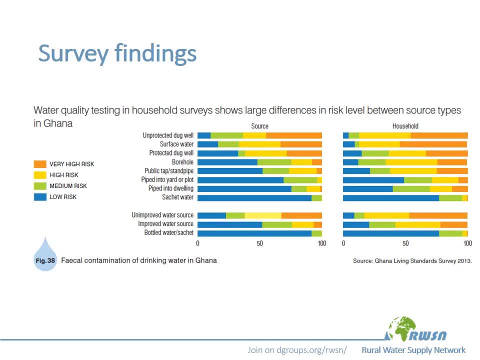 One of the key advantages of integrating water quality testing in a household survey is that you can look at water quality and risk levels by all of the characteristics included. 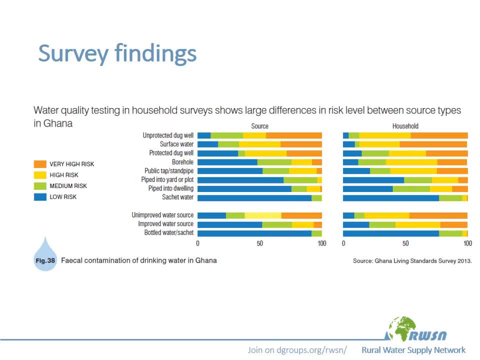 So, for example, here we're just showing risk levels in Ghana for the source and the household for different main sources of drinking water. And what we can see is that there's, as we would expect, a big difference between unprotected dug wells and piped water into dwelling and sachet water. 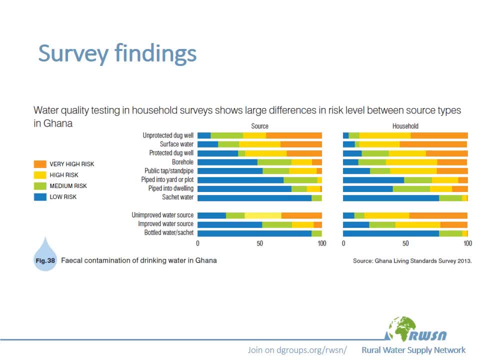 So. The blue low risk is much higher for those categories. And in almost all cases, we see a deterioration between the source and the household. 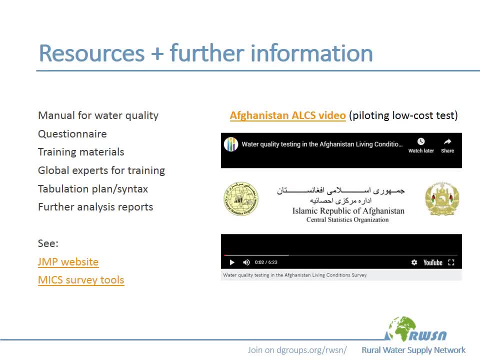 If you want to find out more about the module, I'd really encourage you to have a look at some of the resources. So, for example, the manual for water quality, which describes all of the steps, the questionnaire that we've been using. And you can find those on the mixed survey tools. 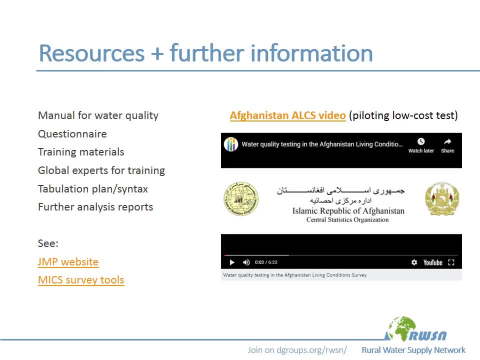 And there's also further information about the different surveys and the final reports on the JMP website. 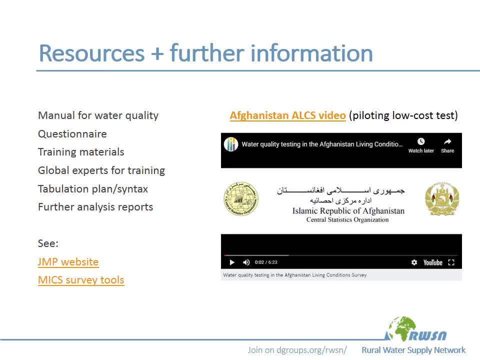 There's also a very neat video that was produced by Central Statistics Organization of Afghanistan, which shows a pilot using a lower cost manifold and a phase change incubator. 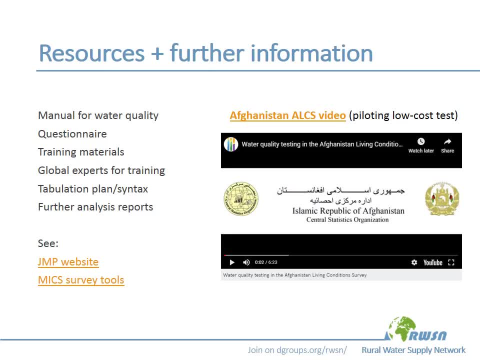 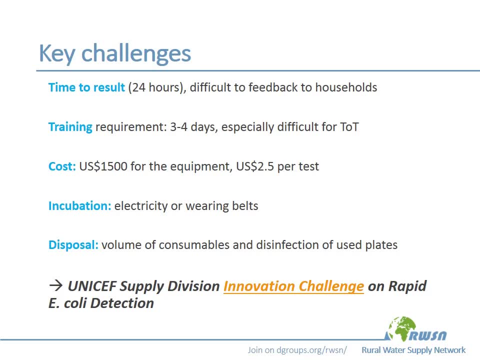 So there's a video there that you can have a look at too. There are a number of key challenges associated with water quality testing and household surveys, just as much as they may be also in regular monitoring. So, for example, here, time to result. Because nearly all tests are based on culture, they require 24 hours incubation. 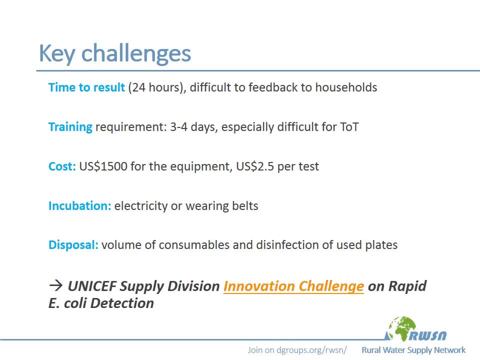 And that means that we find it very hard to provide feedback to households. 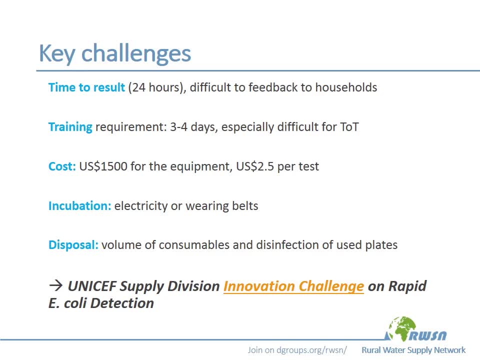 Training for member infiltration usually takes about three to four days for people who don't have previous experience. And that's especially difficult if you're trying to cascade training through your training of trainers. 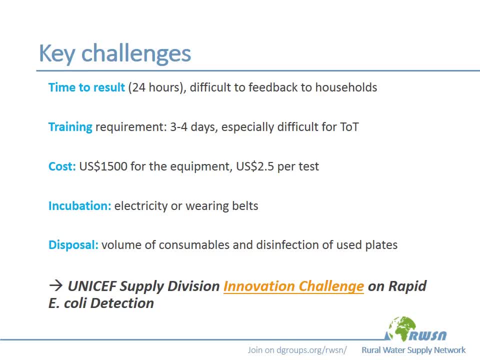 And the cost of the equipment is about $1,500 per team and $2.5 per test. 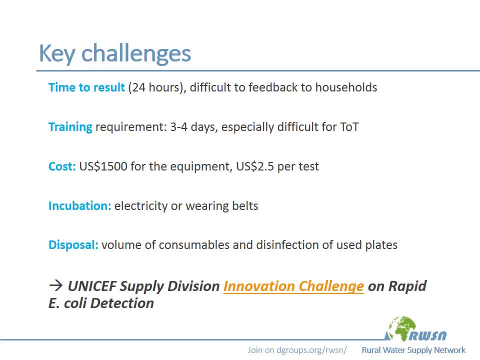 And we're looking at ways to reduce that cost. Incubation, difficult to persuade teams to wear belts at night. 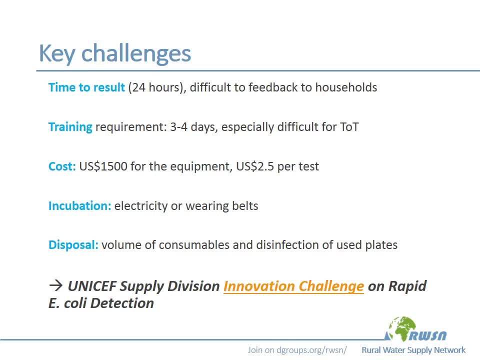 And it's also particularly difficult in countries where that might be perceived as a security risk. Disposal, there's lots of consumables in this testing approach. 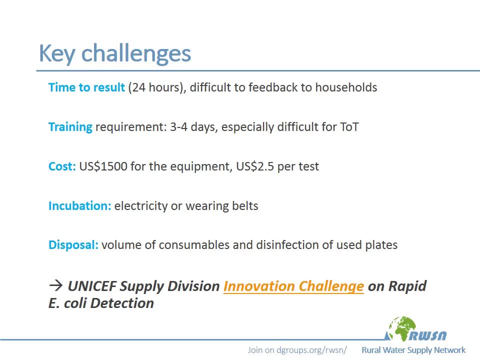 And together with UNICEF's supply division, we've launched an innovation challenge to look at ways to come up with more rapid care light tests and to encourage manufacturers to devise those. 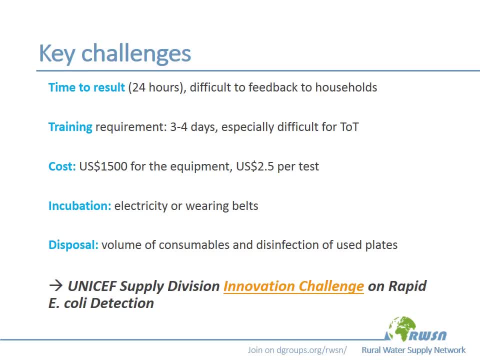 So hopefully in the next few years, we'll be able to adopt those and adapt the module accordingly. 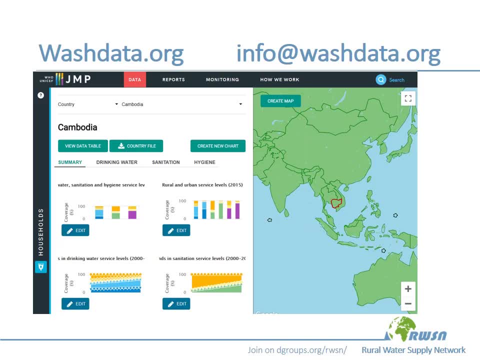 So with that, I'd just like to say thank you for listening. And if you have any questions, please do get in touch with us at info at washdata.org. 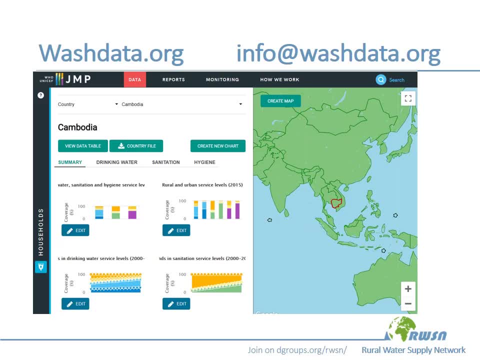 And I'd also encourage you to have a look at the JMP website, which is washdata.org, where you can explore the data for individual countries. 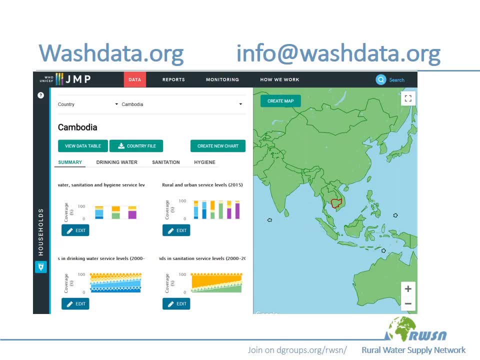 And look at inequalities for households, schools and healthcare facilities.